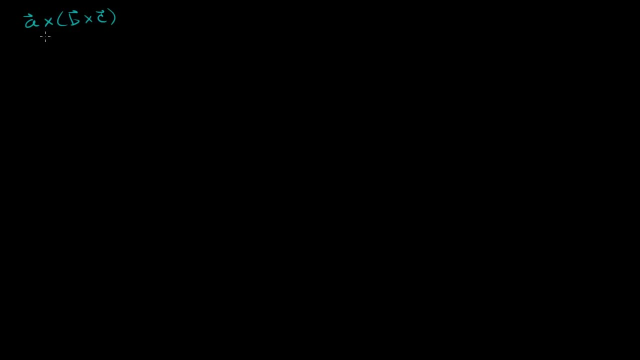 can express this. we can express this really as sum and differences of dot products. well, not just dot blocks, dot products, scaling different vectors. you're going to see what I mean. but it simplifies this expression a good bit, because cross products are hard to take. they're computationally intensive. 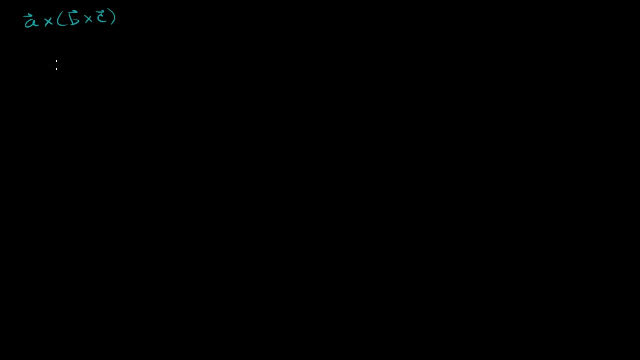 and, at least in my mind, they're confusing. now, this isn't something you have to know if you're going to be dealing with vectors, but it's a useful to know. I my motivation for actually doing this video is I saw some problems for the Indian institute of technology entrance exam. that seems. 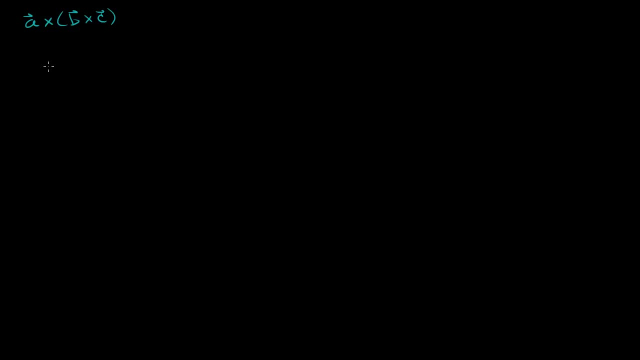 to expect that you know Lagrange's formula or the triple product expansion. so let's see how we can simplify this. so to do that, let's start taking the cross product, let's start taking the cross product of b and c, and in all of these situations- I'm just going to assume- let's say a. 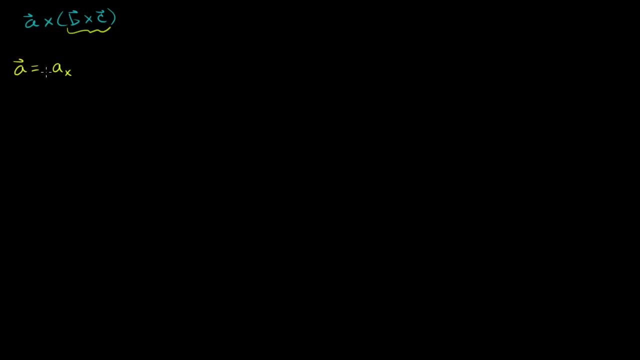 vector a. I'm just going to call that. that's going to be a, the x component of vector a times the unit vector i plus the y component, not b plus the y component of vector a times the unit vector j plus the z component of vector a times unit vector k, and I could do the same things for b and c. so if 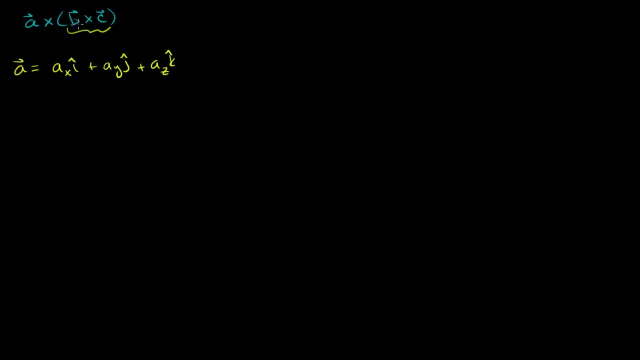 sub y. I'm talking about what, scaling the j component in the b vector. so let's first take this cross product over here, and if you've seen me take cross products, you know that I like to do these little determinants and what. let me just take it over here. so b cross c, b cross c is going. 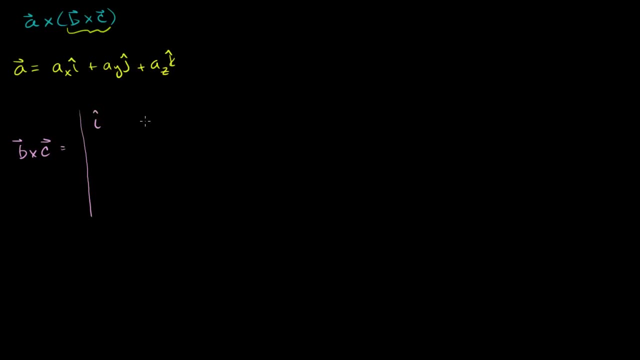 to be equal to the determinant, and I put an i j k up here: i j k. this is actually the definition of the dot product. sorry to show you why this is true. this is just one way to remember the dot product if you remember how to take determinants of three by threes, and we'll put b's x term, b's y coefficient. 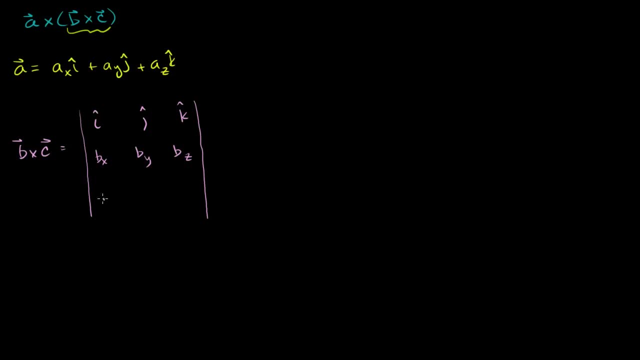 and b's z component, and then you do the same thing for the c, cx, cy, cz, and then this is going to be equal to. so: first you have it's the i component, so it's going to be the i component times to ignore this column in this row. so BYCZ minus BZCY. 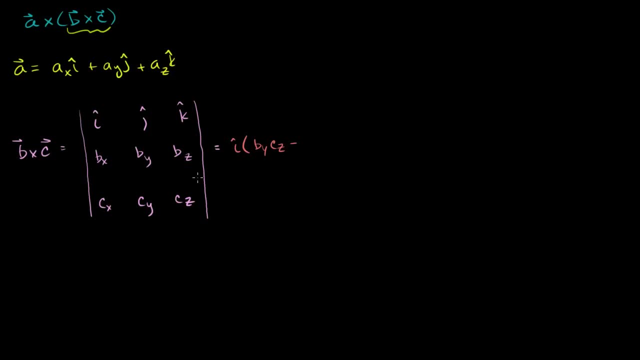 So I'm just ignoring all of this and I'm looking at this 2 by 2 over here, minus BZCY, And then we want to subtract the j component. Remember we alternate signs when we take our determinant. Subtract that, and then we take out that column and that row. 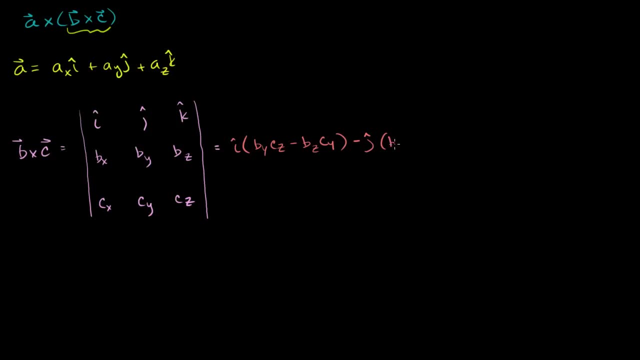 So it's going to be BXCZ. this is a little monotonous, but hopefully it'll have an interesting result: BXCZ minus BZCX And then finally, plus the k component k, we're going to have BX times CY minus BYCX. 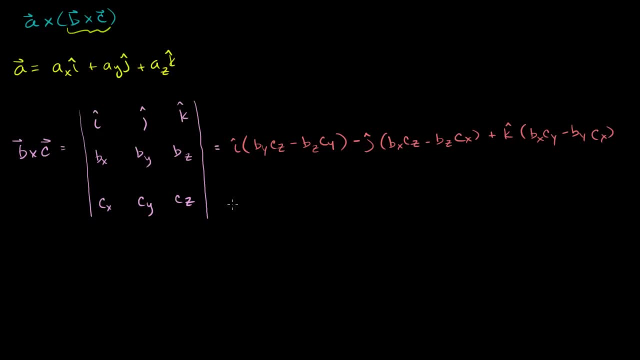 So this is: we just did the dot product And now we want to take the. oh sorry, we just did the cross product. I don't want to get you confused: We just took the cross product of B and C And now we need to take the cross product of that with A. 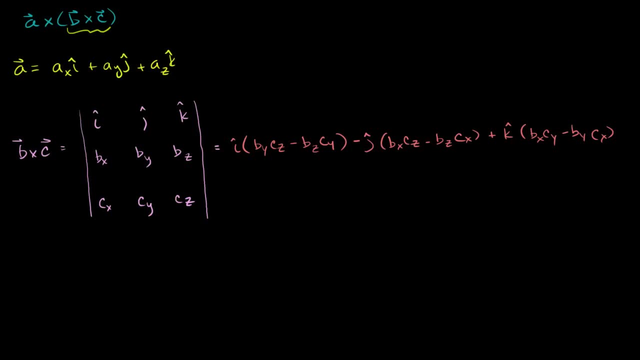 or the cross product of A, with this thing right over here. So let's do that Instead of rewriting the vector. let me just set up another matrix here. So let me write my IJK up here: IJK, IJK, IJK. 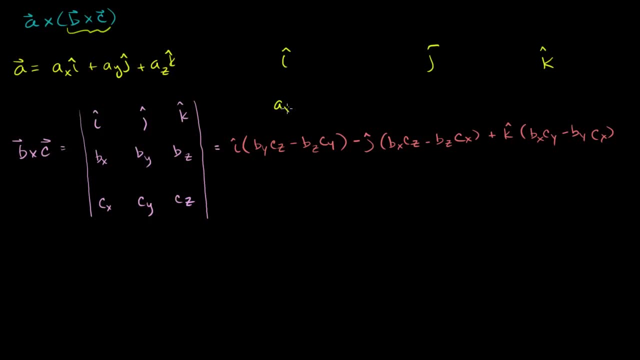 IJK, IJK, IJK, IJK. And then let me write A's component, So we have A sub X, A sub Y, A sub Z, And then let's clean this up a little bit. Let's ignore this. 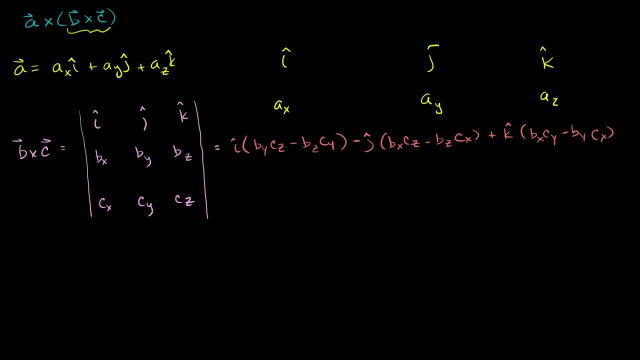 We're just looking at. I want to do that in black. Let's do this in black so that we can kind of erase that. Now, this is a minus J times that. So what I'm going to do is I'm going to get rid of the minus and the J. 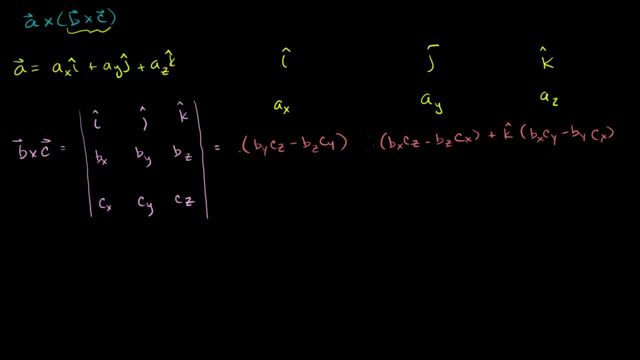 But I'm going to rewrite this with the signs swapped. So this is going to be: if we swap the signs, it's actually BZCX minus BXC minus BXCZ. So let me delete everything else. So I just took the negative and I multiplied it by this. 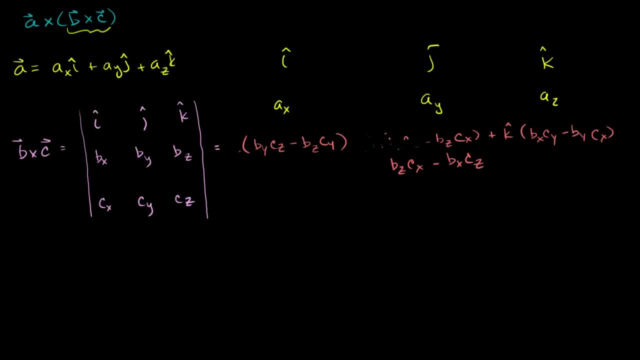 I hope I'm not making any careless mistakes here. So let me just I can make my brush size a little bit bigger so I can erase that a little more efficiently. There you go, And then we also want to get rid of that right over there. 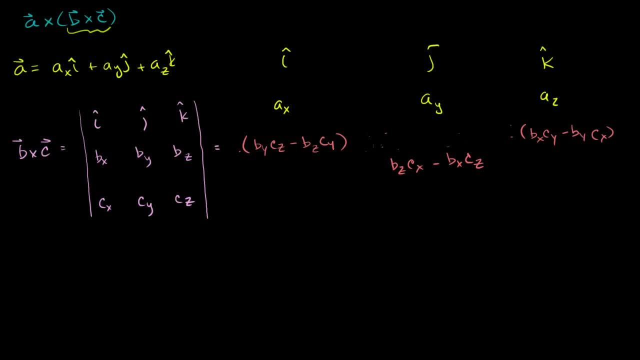 Now let me get my brush size back down to normal size, All right. so now let's just take this cross product, So once again set it up as a determinant, And what I'm only going to focus on, because it'll take the video or it'll take me forever. 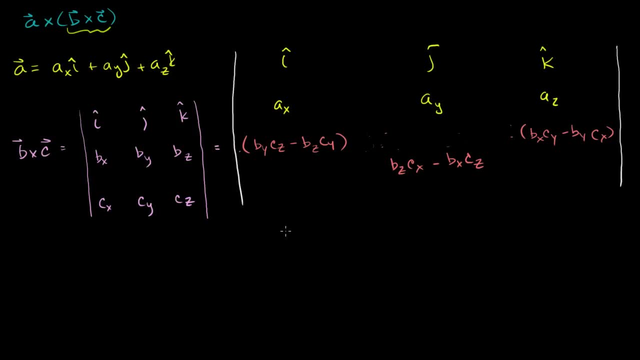 if I were to do the I, J and K components. I'm just going to focus on the I component, just on the X component of this cross product, And then we can see that we'll get the same result for the J and the K. 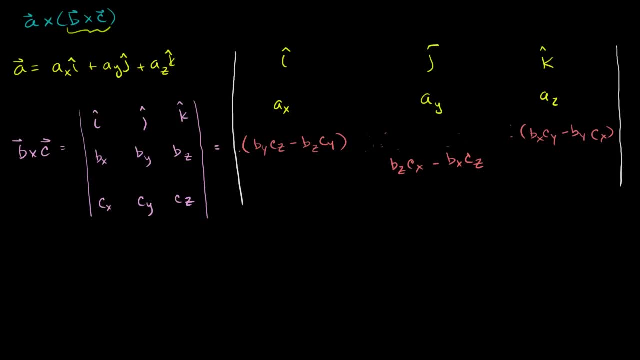 And then we can see what hopefully this simplifies down to. So if we just focus on the I component here, this is going to be I times- and we just look at this 2 by 2 matrix, right over here, We ignored I's column, I's row. 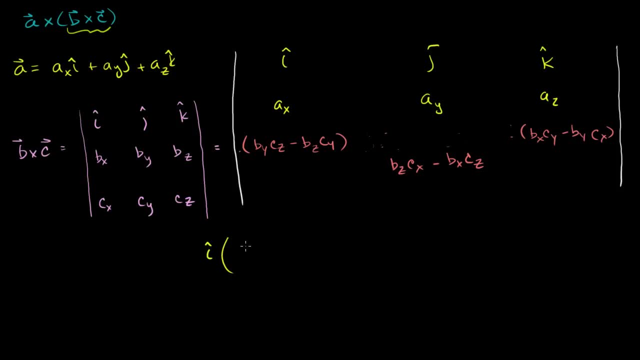 And we have Ay times all of this. So let me just multiply it out. So it's Ay times BXCY Minus Ay times BY times BYCX. and then we're going to want to subtract, We're going to have minus Az times, this. 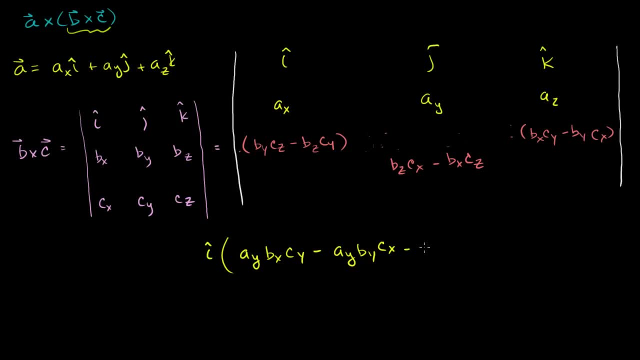 So let's just do that, So it's minus or negative Az BZCX, And then we have a negative Az times this, so it's plus Az BXCX. And now what I'm going to do? this: 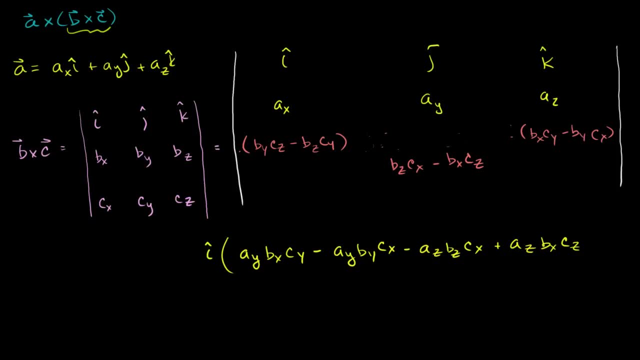 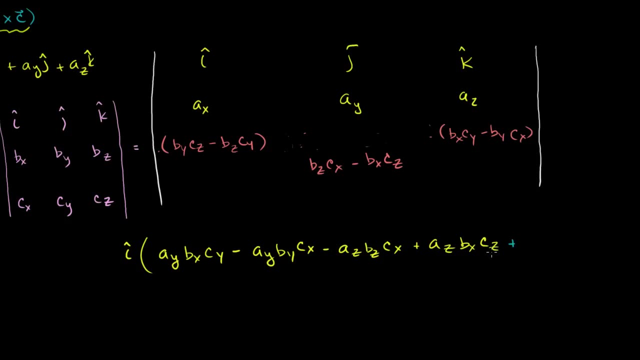 is a little bit of a trick for this proof right here. just so that we get the results that I want, I'm just going to add and subtract the exact same thing. So I'm going to add an AXBXCX and then I'm. 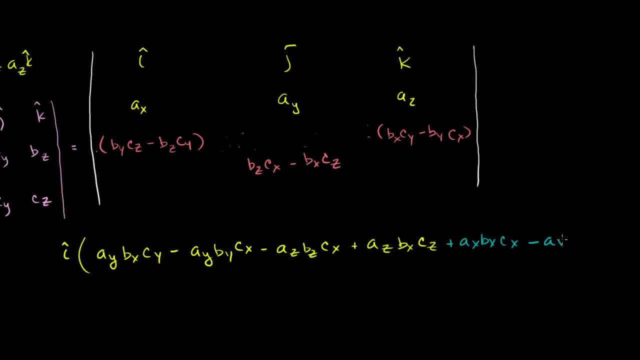 going to subtract an AXBXCX Minus AXBXBXCX Minus AXBXBXCX Minus AXBXBXCX. So clearly, I have not changed this expression. I've just added and subtracted the same thing. 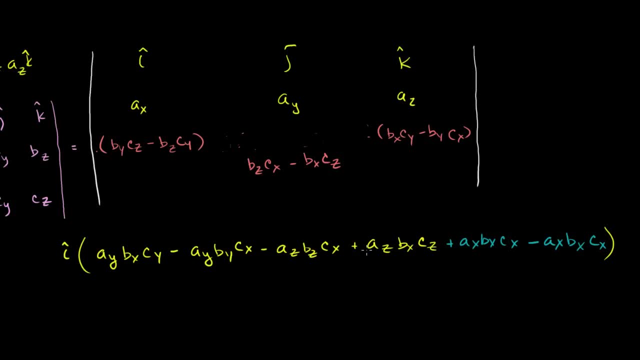 And let's see what we can simplify. Remember, this is just the x component of our triple product, Just the x component. But to do this, let me factor out, I'm going to factor out a BX, So let me do this. 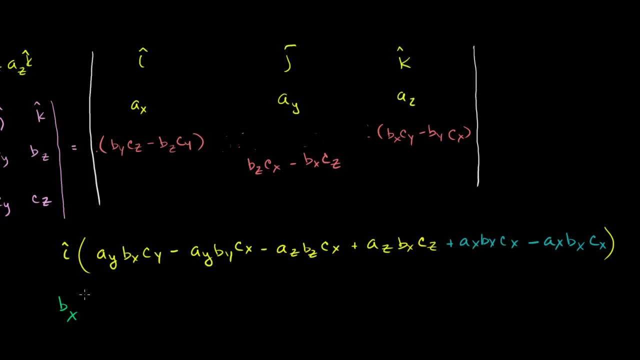 Let me get the BX. So if I were to factor it out and I'm only going to look at, I'm going to factor out of this term that has a BX, I'm going to factor out of this term And then I'm going to factor it out of this term. 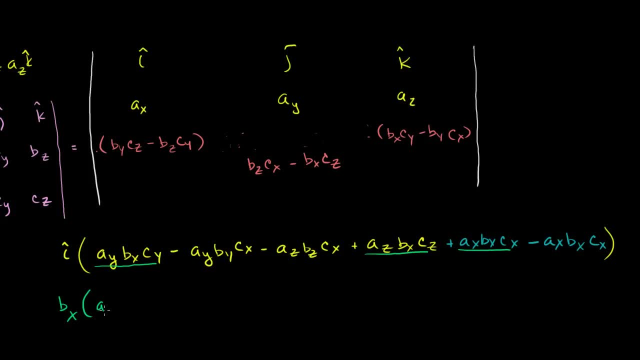 So if I take the BX out, I'm going to have an AYCY. Actually, let me write it a little bit differently. Let me factor it out of this one first. So then it's going to have an AXCX. 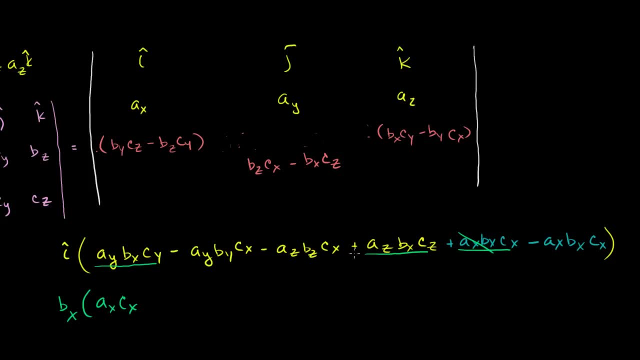 AXCX. So I use this one up And then I'm going to have a. I'll do this one now. Plus, if I factor the BX out, I get AYCX, AYCX, AYCX, AYCX. 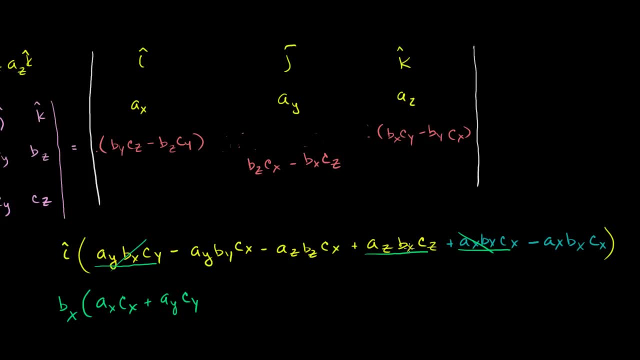 AYCX And C sub Y. I've used that one now, And now I have this one, I'm going to factor the B sub X out, So I'm left with a plus A sub Z, C sub Z. So that's all of those. 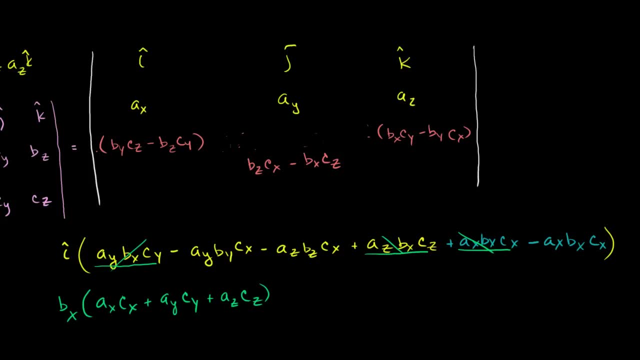 So I factored that out. And now from these right over here, let me factor out a negative C sub X, And so if I do that, let me go to this term right over here. I'm going to have an AXBX when I factor it out. 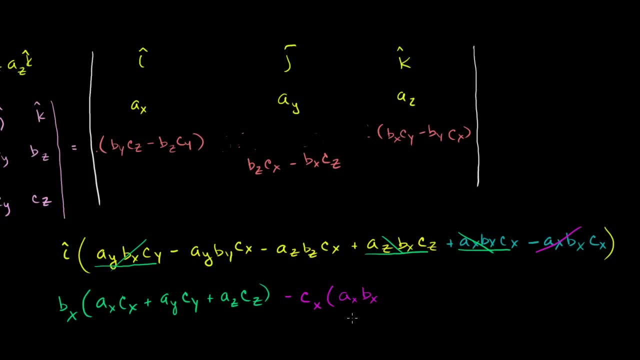 So an AXBX. Let me cross that out. And then over here I'm going to have an AYBY. Remember I'm factoring out a negative C sub X, So I'm going to have a plus A sub Y, B sub Y. 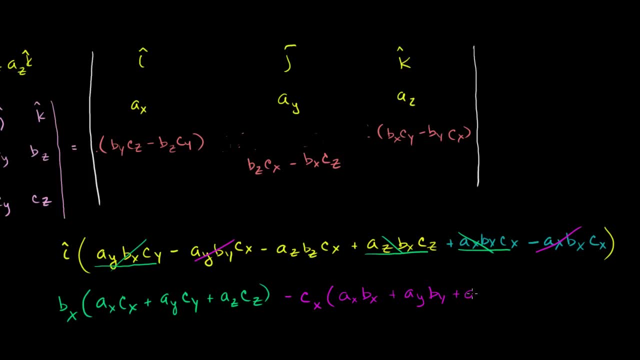 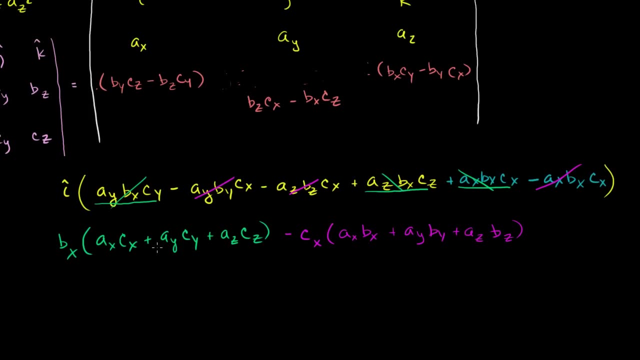 And then, finally, I'm going to have a plus A sub Z, B sub Z. And what is this? Well, this right here in green: this is the exact same thing as the dot products of A and C. This is the dot product of the vectors A and C. 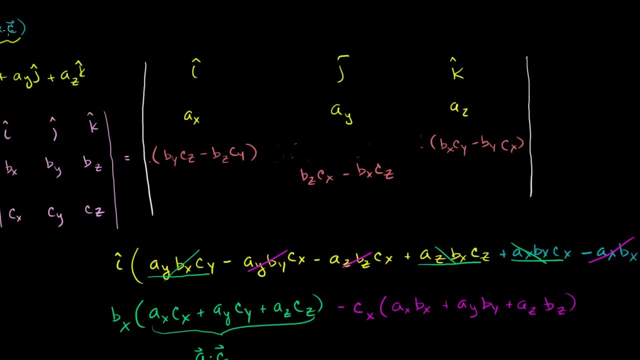 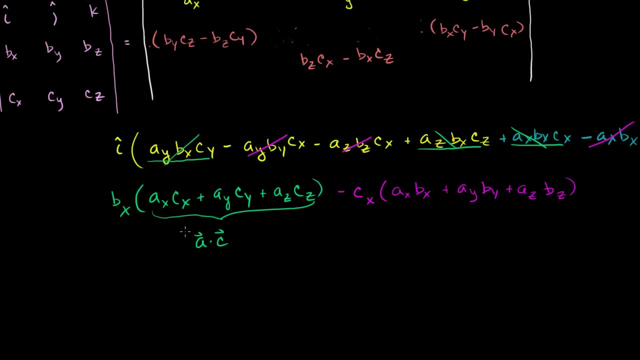 It's the dot product of this vector and that vector. So that's the dot of A and C times the x component of B, minus. I'll do this in the same minus. once again, this is the dot product of A and B. now. 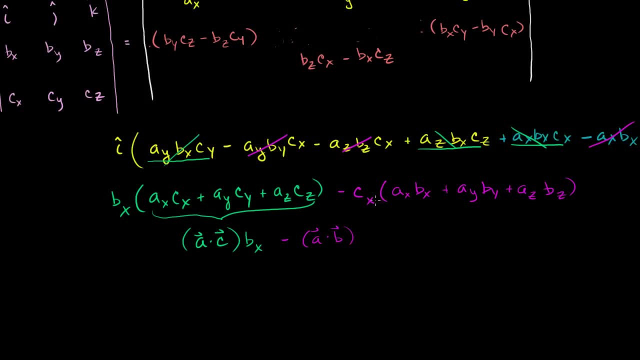 A dot B times the x component of C. And we can't forget, all of this was multiplied by the unit vector i. We're looking at the x component, or the i component of that whole triple product. So that's going to be all of this is times the unit vector i. 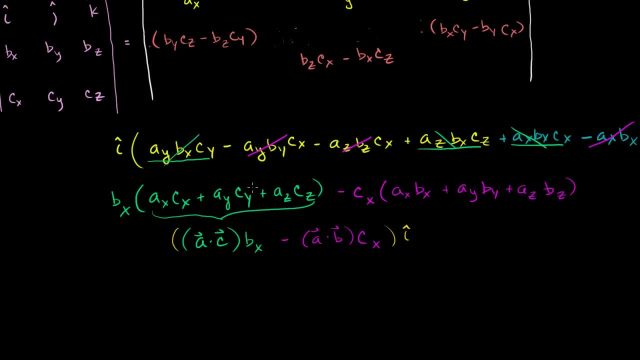 Now, if we do this exact same thing- and I'm not going to do it because it's computationally intensive, But I think it won't be a huge leap of faith for you- This is for the x component- If I were to do the exact same thing for the y component. 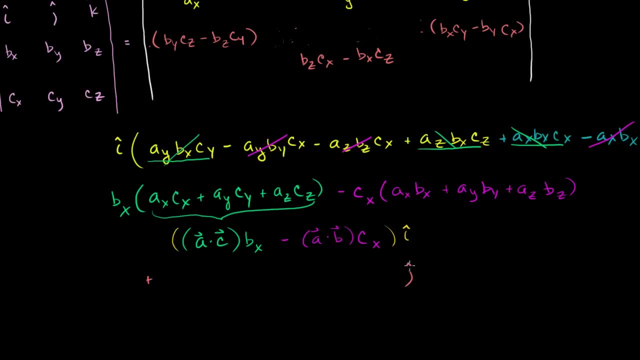 for the j component. so it'll be plus If I do the same thing for the j component. we can really just pattern match. We have B sub x, C sub x, That's for the x component. Well, we'll have B sub y and C sub y for the j component. 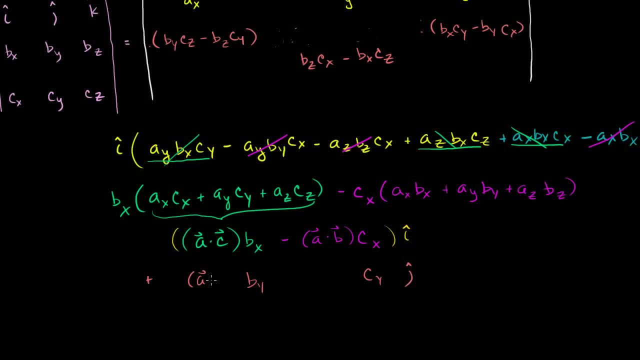 And then this is not component specific, So it'll be A. it will be A dot C over here and minus A dot B over here. You can verify any of these for yourself if you don't believe me, But it's the exact same process we just did. 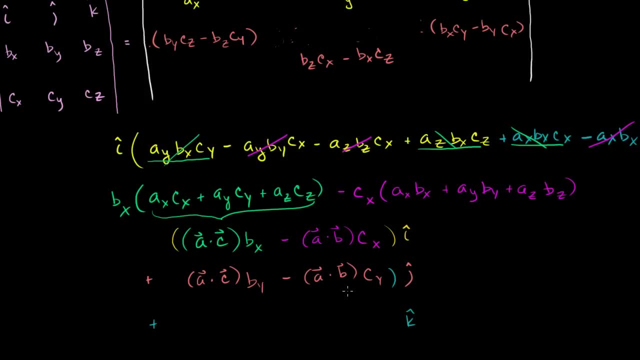 And then finally, for the z component or the k component- let me put parentheses over here- same idea: You're going to have B sub z, C sub z, And then you're going to have A dot B over there, And then you're going to have A dot C over here. 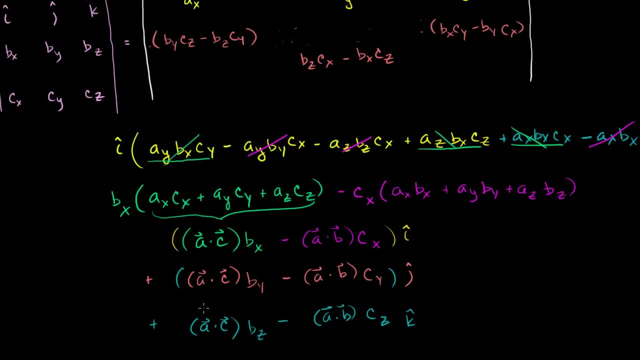 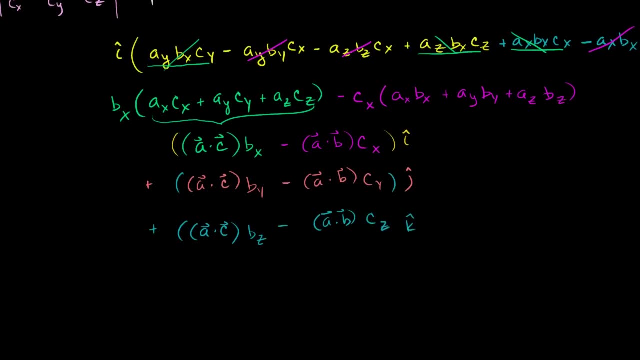 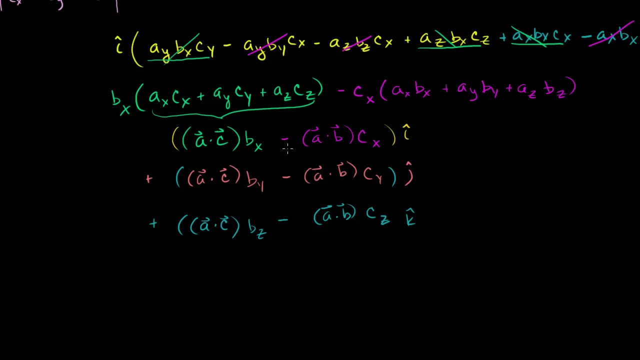 Now, what does this become? How can we simplify this? Well, this right over here, we can expand this out, We can factor out an A, dot, C from all of these terms over here And remember, this is going to be multiplied times i. 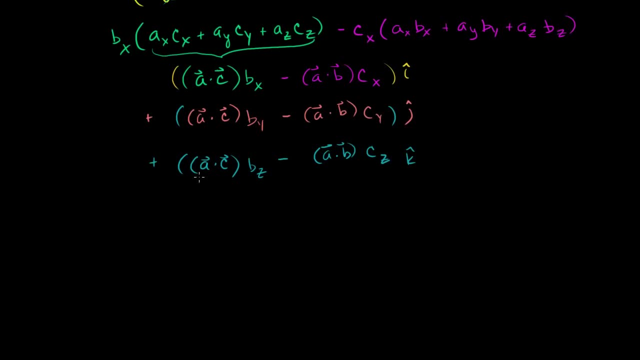 Actually, let me not skip too many steps just because I want you to believe what I'm doing. So if we expand the i here, instead of rewriting it, let me just do it like this. It's a little bit messy, Let's do this here. 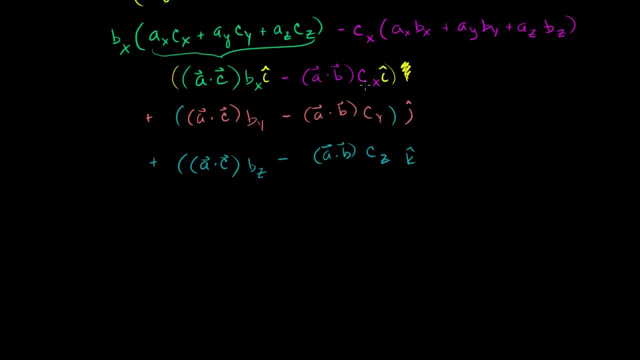 So I could write this i there and that i there. I'm kind of just distributing that x unit vector or the i unit vector. And let me do the same thing for j, So I could put the j there And I could put the j right over there. 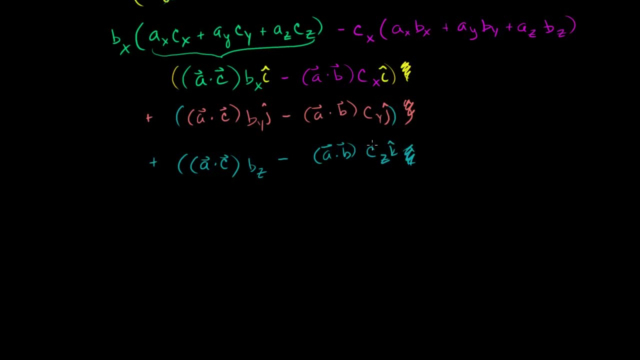 And then I could do the same thing for the k: Put the k there, And then put the k there. And now, what are these? Well, this part right over here, This is exactly the same thing as A dot C times. 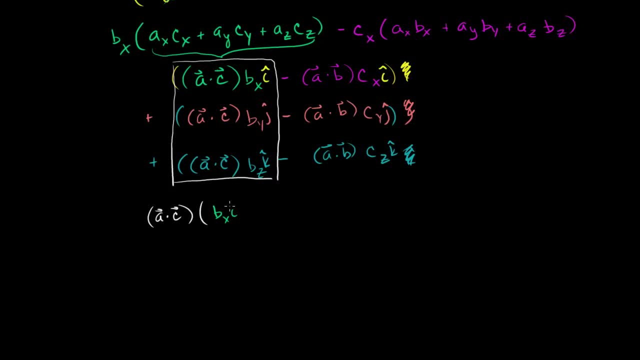 and I'll write it out here: b sub x times i plus b sub y times j plus b sub y times. j plus b sub z times k, And then from that we're going to subtract all of this: A dot B. We're going to subtract A dot B times, the exact same thing. 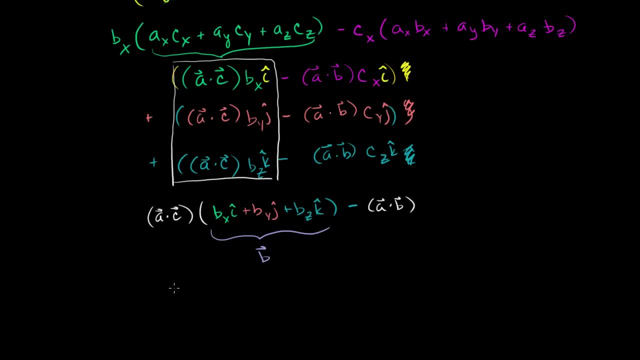 And you're going to notice this right: here is the same thing as vector B. That is vector B. When you do it over here, you're going to get vector C. So I'll just write it over here: You're just going to get vector C. 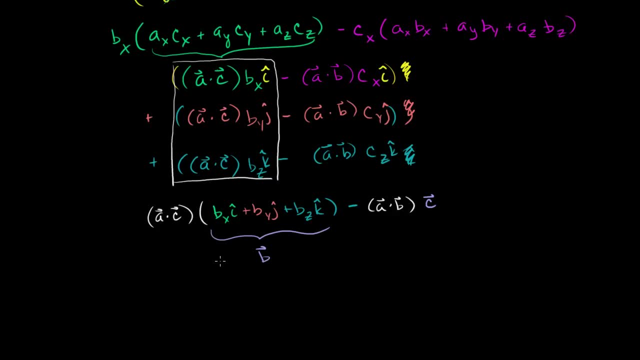 So just like that, we have a simplification for our triple product. I know it took us a long time to get here, But this is a simplification. It might not look like one, But computationally it is. It's easier to do. 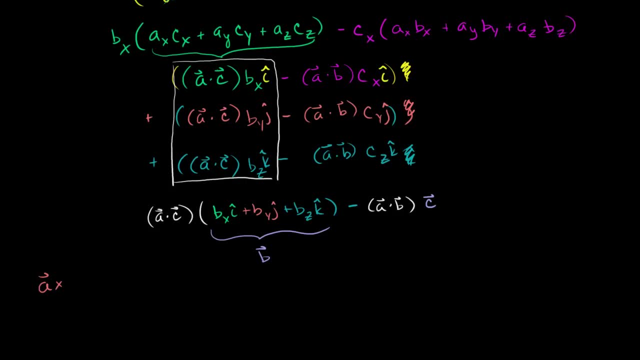 If I have, I'll try to color code it: A cross B, cross C. we just saw that this is going to be equivalent to, and one way to think about it is it's going to be: you take the first vector times the dot product. 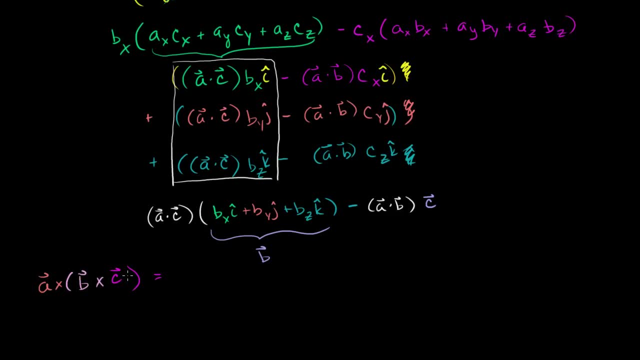 of the first vector in this second dot product, the one that we have our parentheses around, the one we would have to do first. You take your first vector, You take your first vector there, So it's vector B, And you multiply that times the dot product. 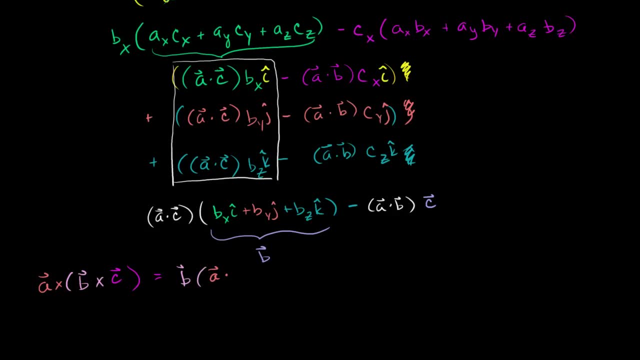 of the other two vectors, So A dot C, And from that you subtract the second vector multiplied by the dot product of the other two vectors of A dot B, And we're done. This is our triple product. This is our triple product expansion. 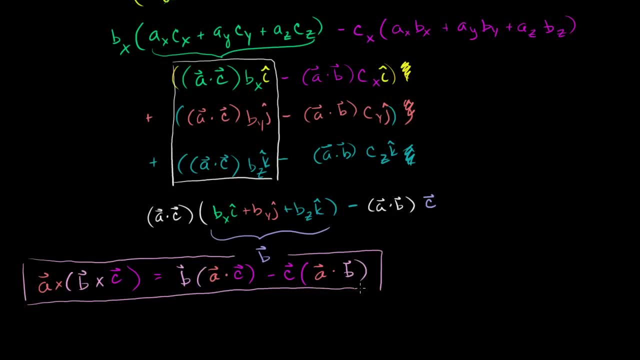 Now, once again, this isn't something that you really have to know. You could always, obviously, multiply it. You could actually just do this. You could do it by hand. You don't have to know this, But if you have really hairy vectors,